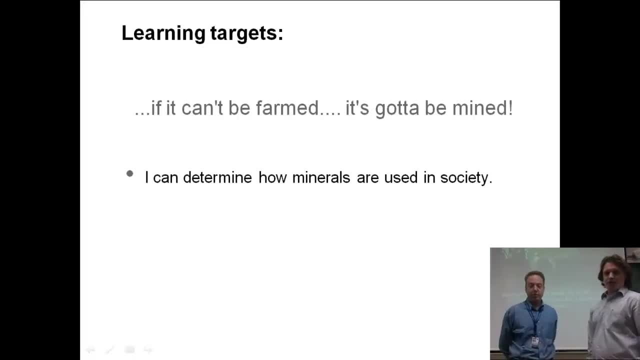 It's going to be a long one. I think I'm excited, though. Yeah, I am too. Let's see what we've got. We've got some learning targets. One of the sayings that they have is: if it. 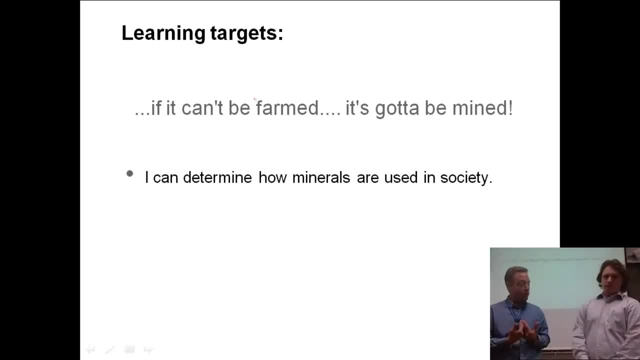 can't be farmed, it's got to be mined. Like what you said, we take things from the earth, things that we need. As geologists, we can tell where to find those things, and those are things that we need to make our world the way that it is. Yeah, and if we just think, 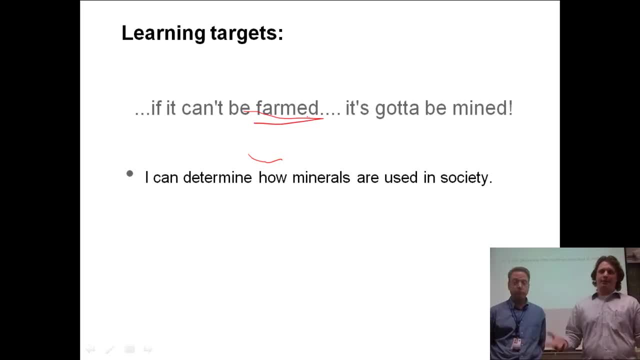 something really simple like our classroom, right? If we look at all the cabinets, they're made out of wood, so that's obviously farmed, right, But everything that we have is farmed. Everything that isn't, I guess, had to come from the ground somewhere, Definitely, yeah. 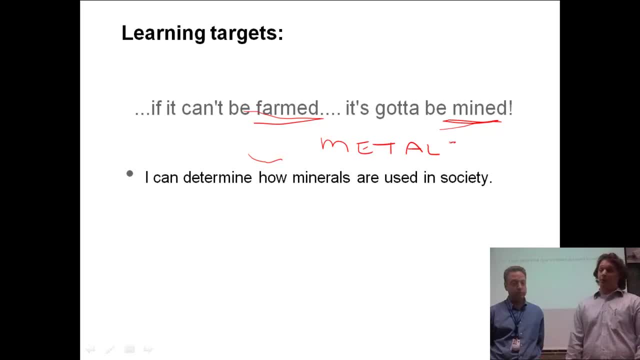 And then there were other things that were used to help produce that that also came from the ground, All right, So that was mined by somebody. So a lot of stuff, a lot of things that probably we don't really think about, or at least take for granted every time. So 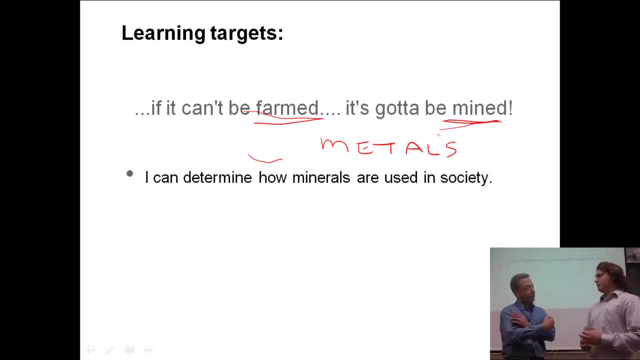 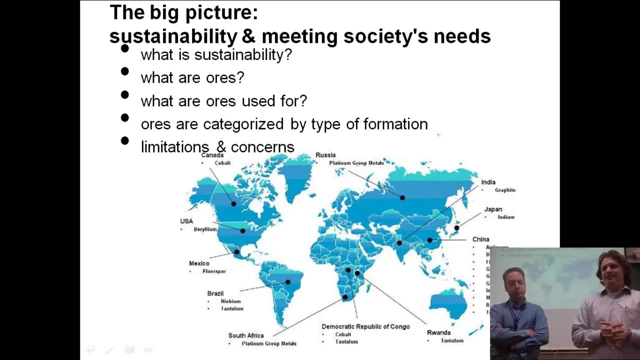 we should be able to determine how minerals are actually used in society. like that, making things? Yeah, definitely, Let's see what we've got. All right, All right. so the big picture is sustainability and meeting society's needs. So what we're going to talk about and this: 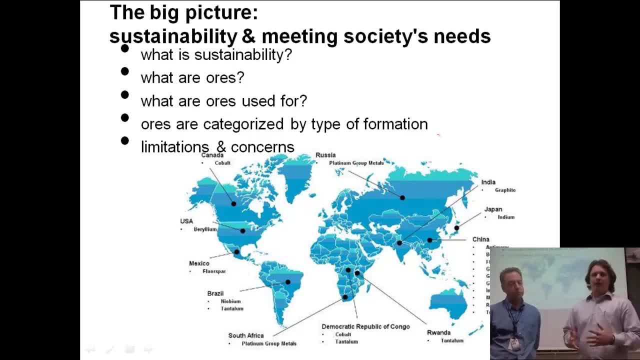 is kind of like an extension of the learning targets are: what is sustainability? what are ores? what are ores used for? ores categorized by type of formation, and then limitations and concerns, And this is almost what we're going to talk about through the entire like. 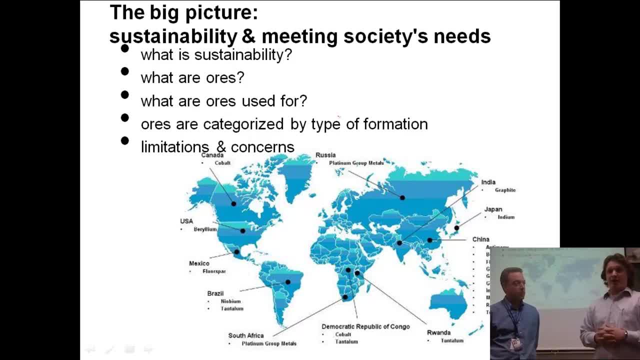 four segments of this, of this, of economic geology. So we've got some words we're going to be learning like sustainability, kind of a balance. you know ores that have to do with the metals themselves and the And the rock. So let's see what we've got coming up here. 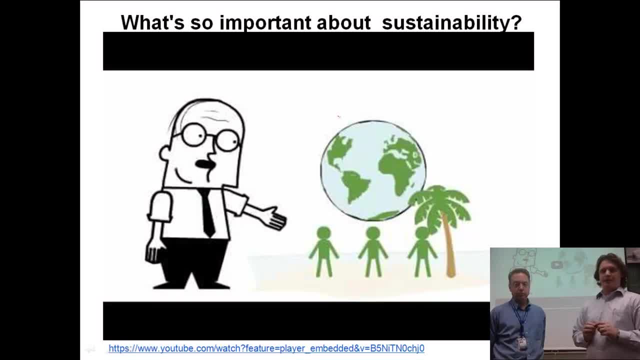 All right. so we do have a video. that is a video in the video about sustainability. So we're going to go ahead and just play this for you right here in the slideshow. So I'm going to go ahead and do that right now. 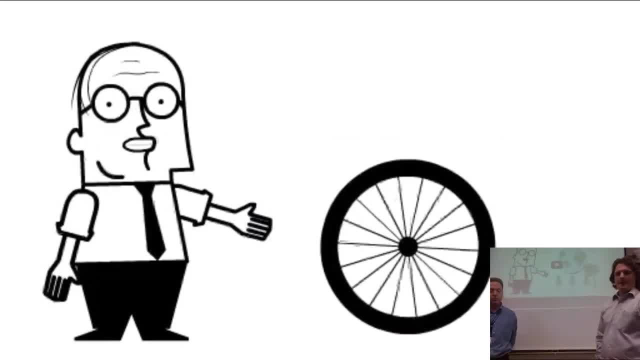 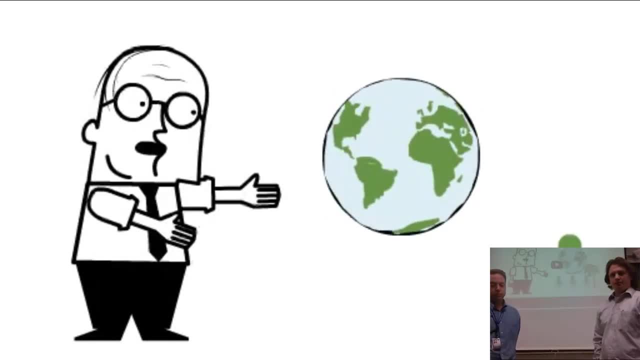 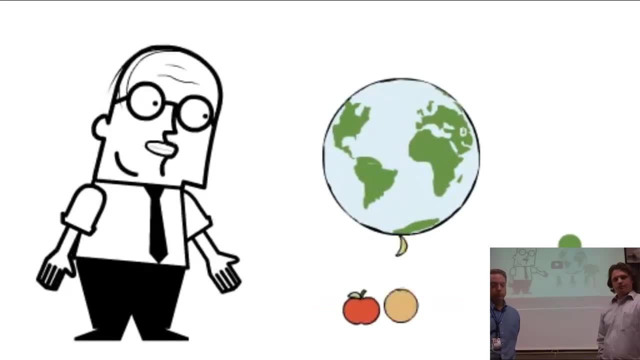 Sustainability means that things can keep going, can sustain themselves, can continue into the future and go on forever. Sustainability for our planet means that it can continue to do what it was designed to do: provide fresh air, clean water, produce food and allow us all to have a high quality. 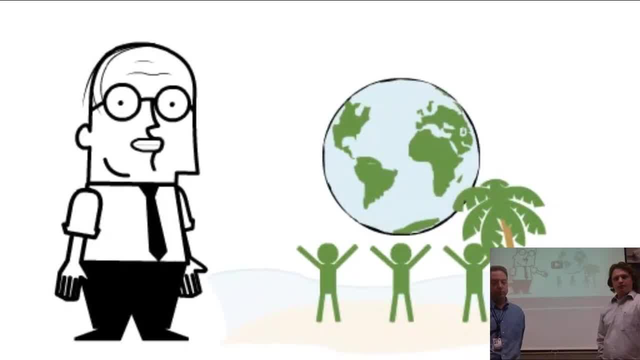 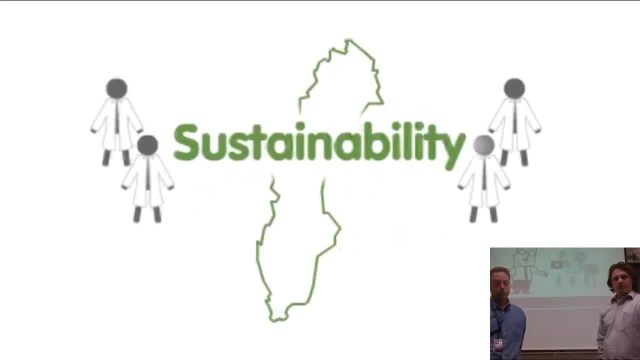 of life forever. Unsustainability means that it cannot, and that is where we are now. Twenty years ago, scientists in Sweden developed a definition for sustainability with four basic principles. These can be seen as the care instructions for our planet If we follow. 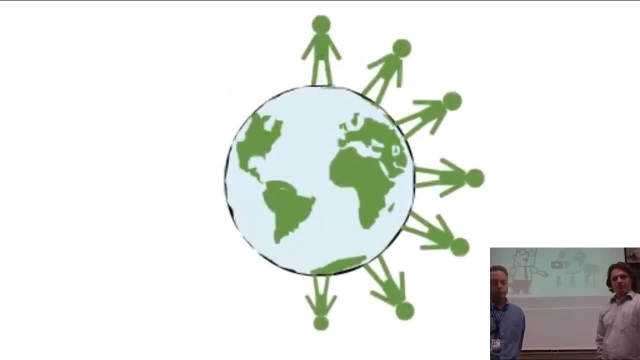 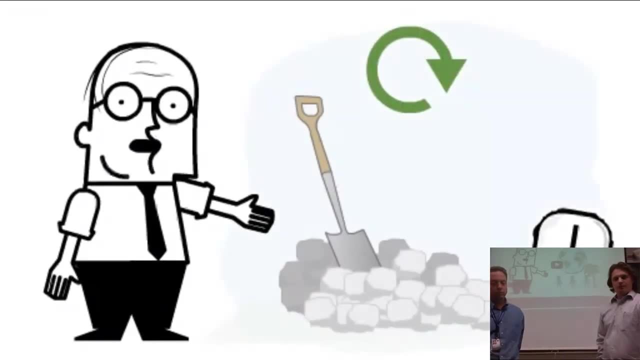 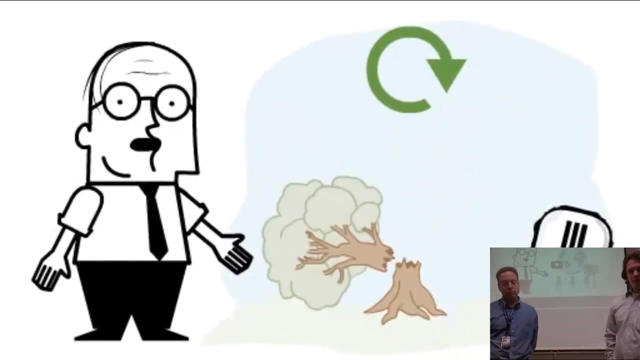 them. it is good for our planet And because we're part of the system that is our planet, it's good for us too. The care instructions are as follows: Reduce our dependence on fossil fuels and heavy metals. Reduce our dependence on synthetic chemicals that persist in nature. Reduce our destruction. 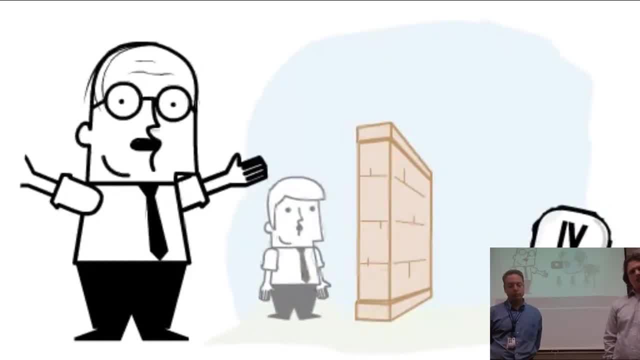 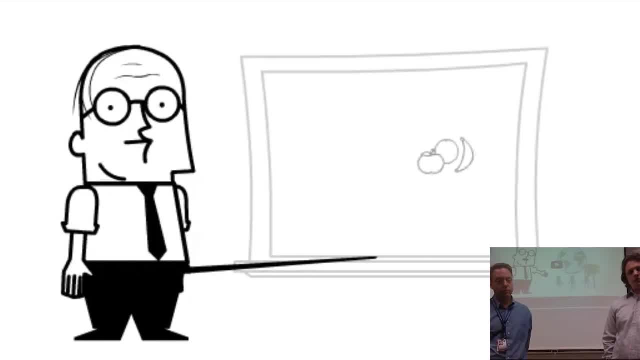 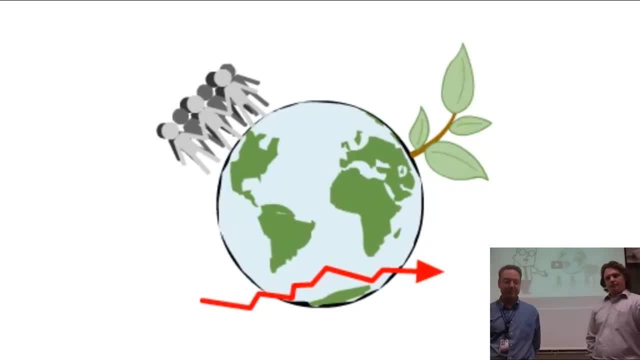 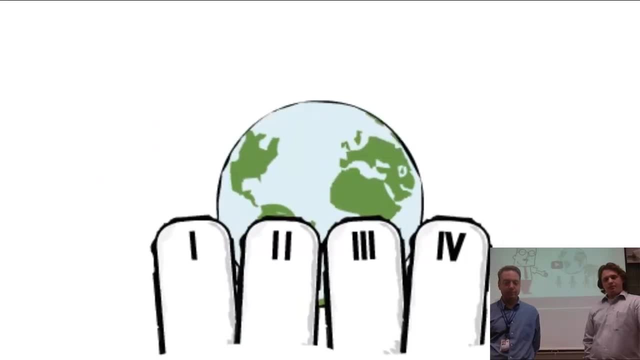 is connected: Society, environment and economy. To live sustainably, we need to follow the four care instructions and apply them to everything we do at home and at work. If we can follow these care instructions, we can work together to be sustainable, We will. 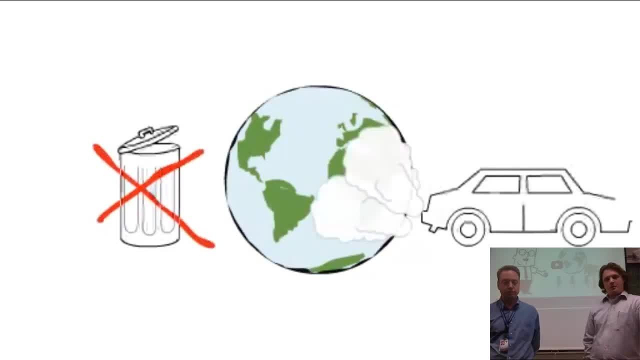 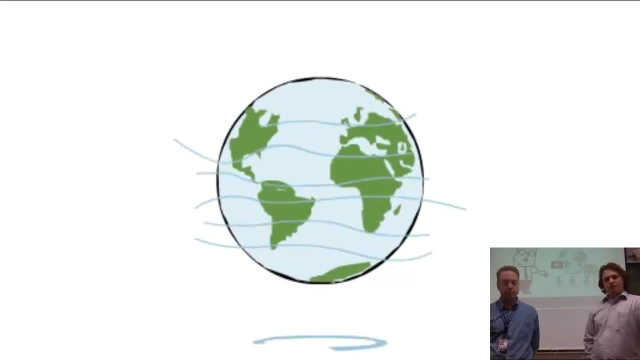 all have a better quality of life. We'll waste less, we'll pollute less and we'll create more things we value in society, while improving our planet's chances of providing us with the very things we need to survive. all right, so that was actually a really good video on. 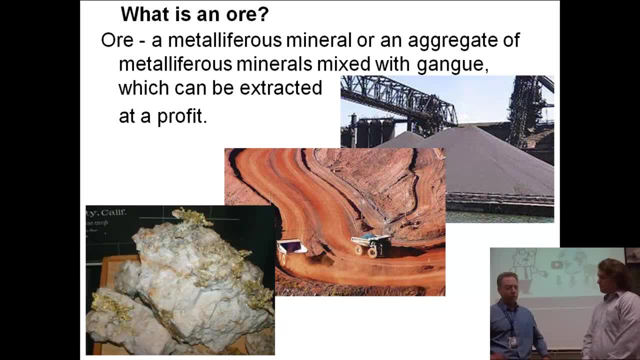 sustainability, don't you think? yeah, i think the main ideas they take away from it is: we're on the earth, we're part of the earth, and so if we're going to take something from the earth, we have to make sure that we don't adversely affect everything that's associated with. yeah, and we. 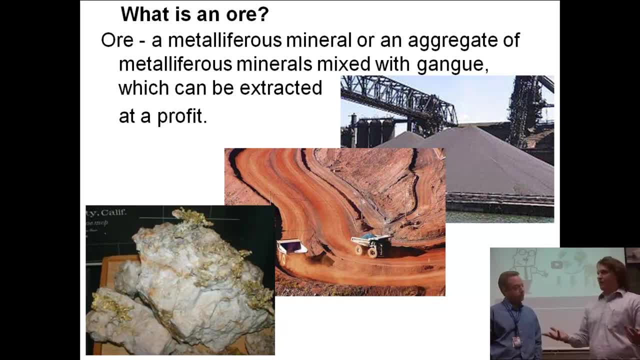 can see a lot of that as a part of, uh like, just in our classroom with like a recycling bin, right, and then you know, like 10 years ago maybe that wasn't around, or 15 years ago wasn't around our classrooms, just to have that kind of idea that we have to kind of be responsible people in terms 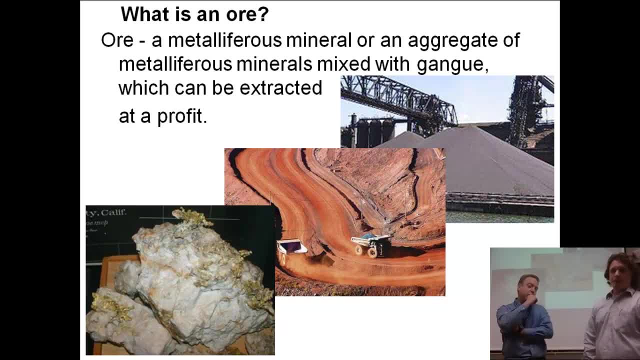 of our environment and what we use and how we use it. okay, so when we go over this, if we throw a few extra words in here that aren't on their slides, they should write a few of that. yeah, definitely. so we are still writing stuff down, definitely, mr z. what is an ore? well, an ore is a metalliferous 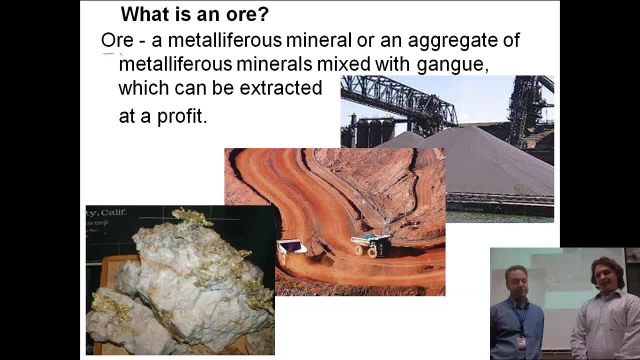 mineral or aggregate of a metalliferous mineral mixed with gang which can be extracted, uh, at a profit. okay, so what does that mean in english terms? okay, well, when we were doing um, the segment, um before with the minerals, the kids scratched something and and the the you had a ore like copper and it was stuck. 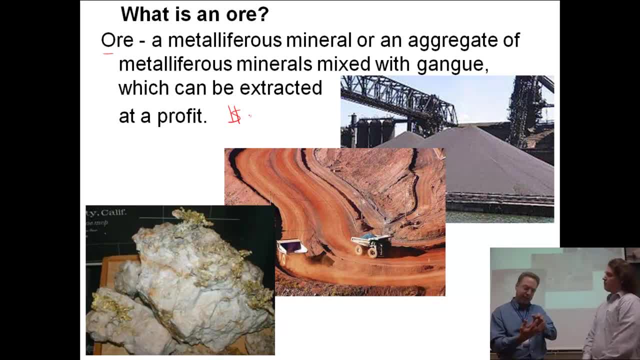 in a bunch of like quartz or some other um, an aggregate or a mixture of other stuff. so the gang would be, if you took the copper out of this, like rock sure. the stuff that's worth the most money, the stuff you're after that's the copper. 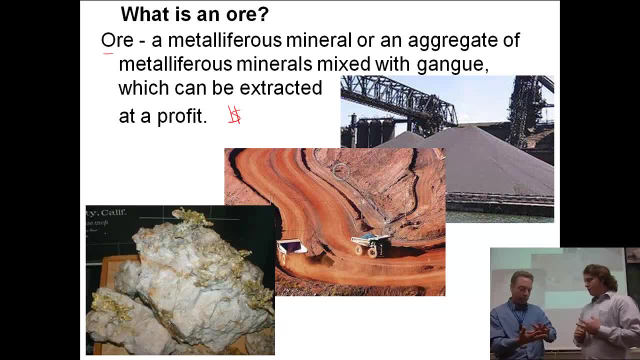 and the gang would be the quartz or the other minerals that it's connected to, an aggregate of minerals that it's stuck to, that doesn't have an economic value to it. so gang is the the stuff that you remove. so the good stuff, the ore, comes out and the gang um kind of goes over there. yeah, 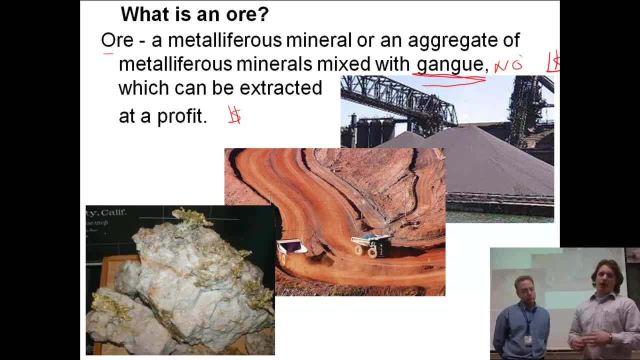 got it and there's a lot of different processes for trying to get that ore out. all right and uh, and basically it's just the stuff that's mixed in with other rocks that we just want and we need to get it out somehow. and the profit is if you can get the gang and the ore separated cheaply enough and then get rid of the. 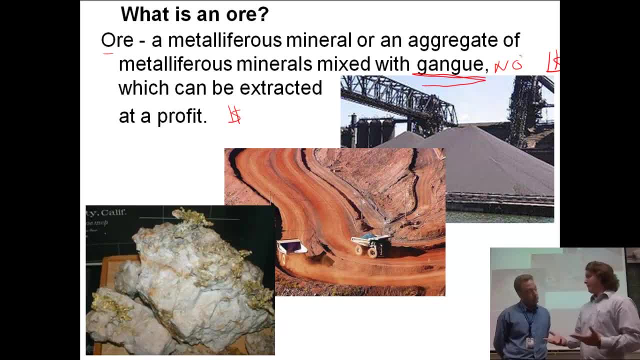 gang and keep the oil. yeah, and if it's not profitable or if it's too expensive to get it out, then it's typically not done, because that's kind of like- uh like- an energy negative. if we have to spend more energy to get out that ore than what we get, then it's not really feasible to do right. 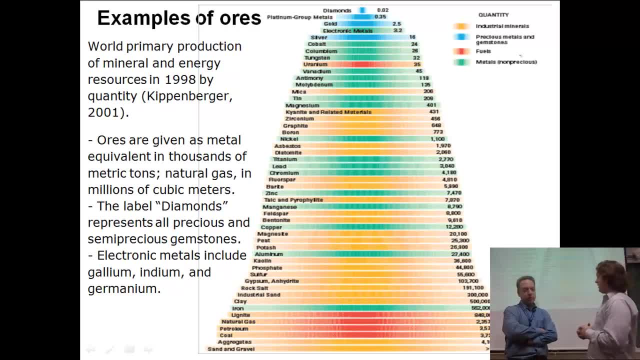 all right. oh, we got a like a pyramid here. so, yeah, that's a huge list, mr man. so these are all things that, um, that it's a world primary production of minerals and energy resources, so these are things that we get out of the ground. um, this would be the things that, um, we're producing, like the minerals. 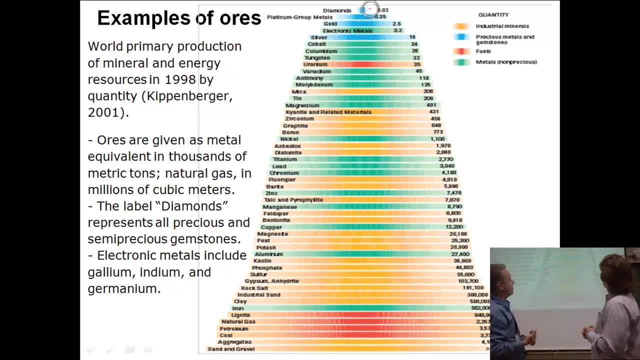 we're producing and as you get near the top, there's what less of them, then, yeah, do you think there'd be value with change as you go up towards the top? yeah, well, i would think that things like sand and gravel- that's all the way down here on the bottom right, it seems like it's pretty abundant. 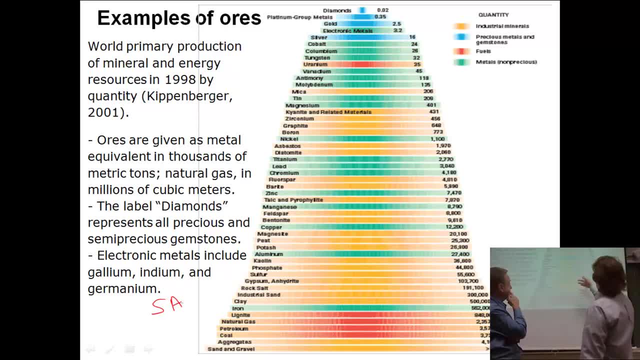 so, um, it's probably pretty cheap, right? so then, if i compare that to diamonds, right, which, if i look over here on the left, is like any precious or semi-precious stone, there's not a whole lot of them, right, so i would think they'd be pretty expensive. so the gist of this slide they should get. 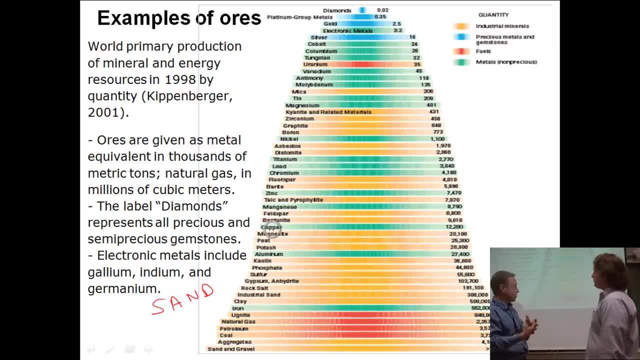 is. these are all things that we take from the earth. they're resources that we need. now, some like here are the big ones. these would be things that we need, and there's a lot of it. maybe it's easy to get the ones at the top. those, um, those. 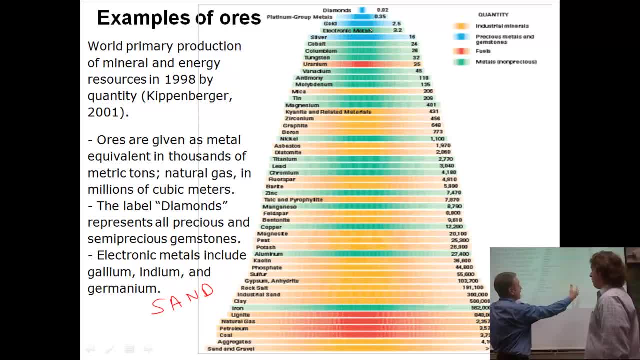 if they were easy to get, they would be really big. so maybe they're not as easy to get, but they're very valuable, yeah, or as plentiful, right? yeah as well. okay, so that's a big list. that is a big list. so we've got yellow is industrial minerals, so anything that's yellow. 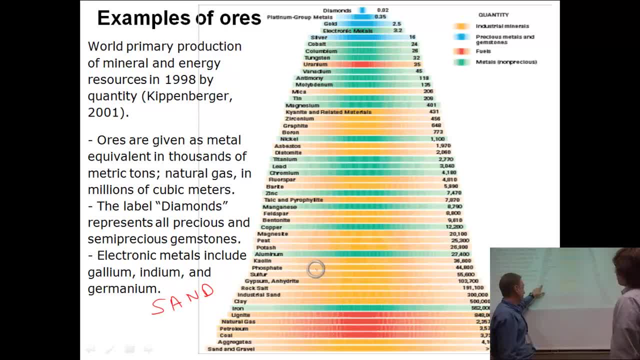 these are things like gypsum board, sulfur, things, that, um, that we're using in industry to make things, and then we've got precious metals and gemstones and, uh, we can see a lot of those up there, but then, oh yeah, they're just all the way up on the top. 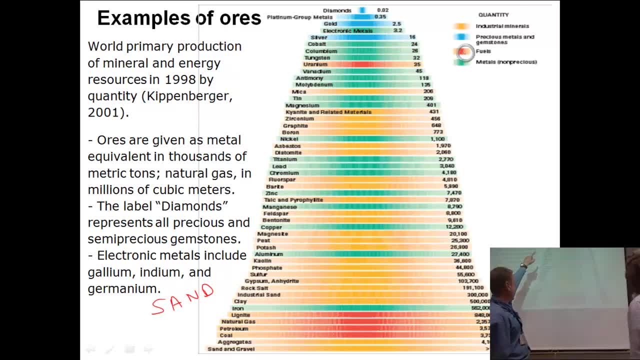 because these are still kind of greenish color, and then we've got fuel, like we've got uranium up there and then some fuel sources down here. so majority of our fuel comes from here, and i guess that makes sense, because this is where you know we're spending a lot of money to produce this, yeah, and 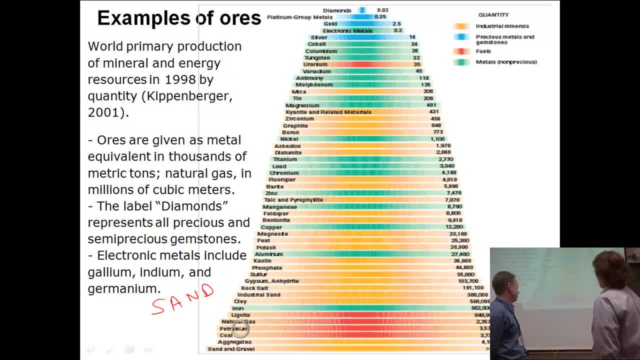 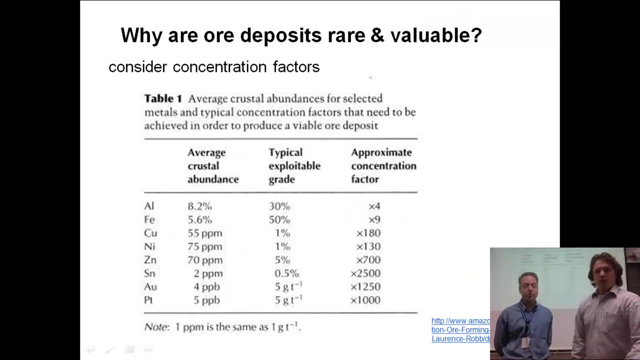 we use this a lot, obviously- natural gas, petroleum- in everyday life for the most part. and then the other thing that we use is our metals. uh, i can't really read that. well, it looks like metals that we use for a variety of other um purposes. yeah, okay, so why are ore deposits and rare and valuable um? so if we're looking at, 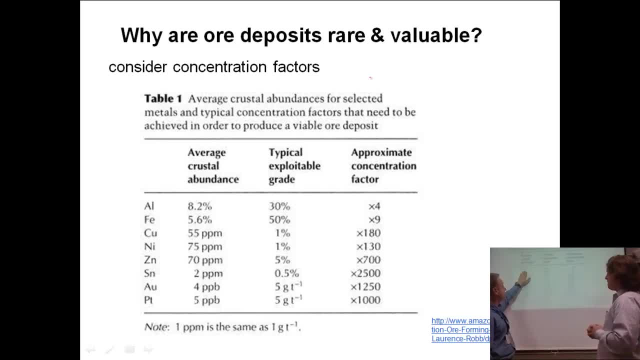 aluminum. typically it sounds like it's about 8.2 percent abundant in the crust. okay, so if you go out and dig a hole just about anywhere, that's average what you would get, but you're not going to make any money unless it's basically what about 30 percent? okay, so there might. 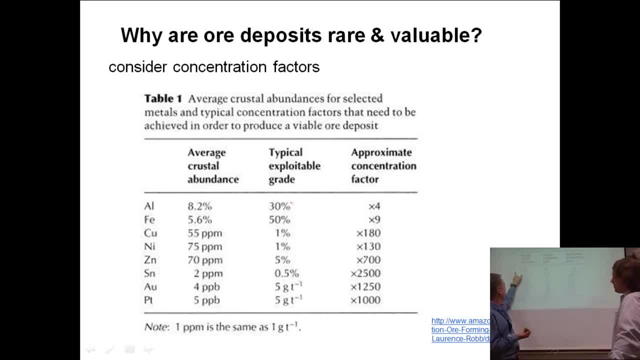 be places. as a geologist, we would know to look where aluminum might have been deposited a long time ago. yeah, because, remember, these are ores, so they're mixed in with other rocks, right? so if we take a rock and it's only eight percent of it is the aluminum inside that rock, then it's we're. 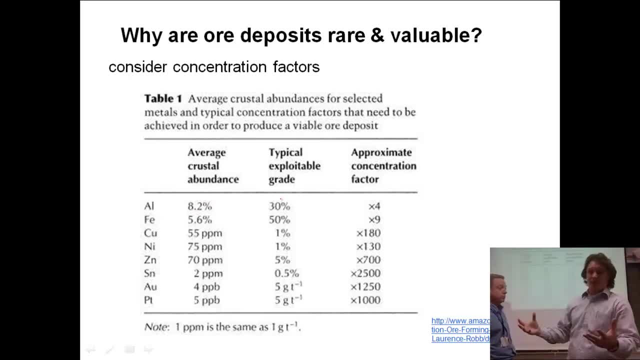 going to be able to separate the ore from the gang or that waste material. and if it's only for this little bit of aluminum, then it's not economically feasible to do. we're just wasting money. so we want to get it to where we have: 30 of that rock is aluminum. then we can continue with that. 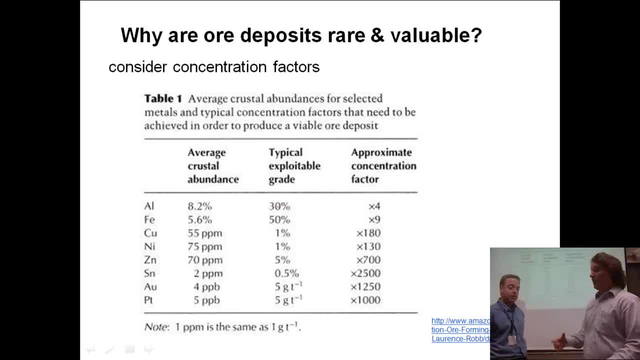 same process to get just more aluminum out. so we want to have that um, that much aluminum in there, and that's the same with with all of these different um metals that we have listed here, and i think this is going to go into that next section where they talk about where we can actually find. 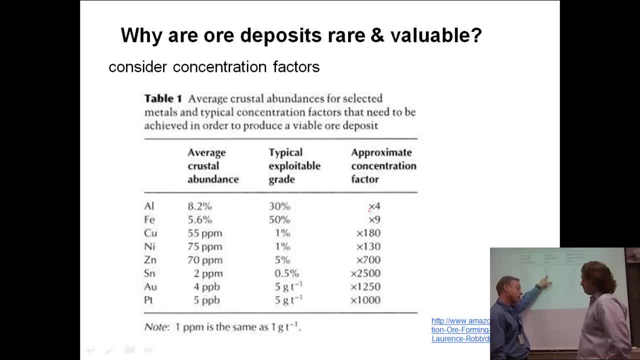 as geologists, where to go looking for things that are really enriched. yeah, and we can talk about that with that tv show too. right, with gold rush, i mean they spend a ton of time and use a lot of resources just to get ounces of gold right, just small, small parts so we can see gold, yeah, right. 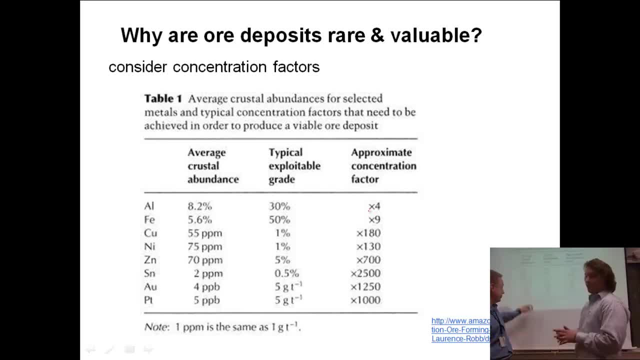 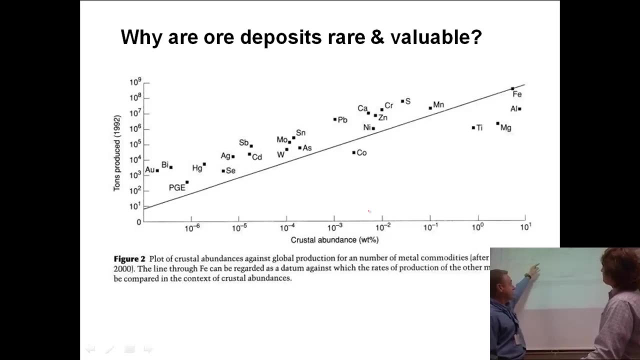 over here. uh yeah, four billion, four parts per billion. so we spend a lot of money and a lot of money on this, and it's very important that we have some stuff that is valuable, all right, so it actually ends up being an economic positive there. okay, so you've got a line here and this line. 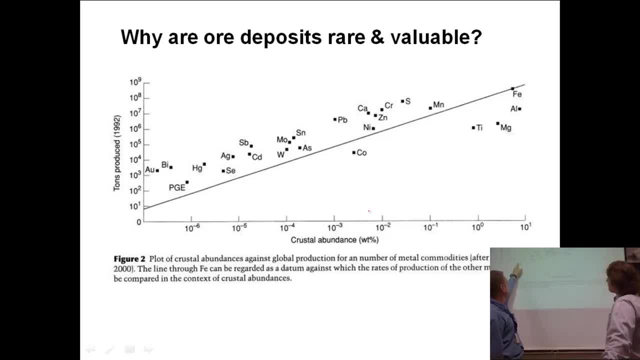 is a very um, like a tipping point line, right, okay, yeah, so anything above the line, these would be things that we would love to have, right? so these would be things that are extremely valuable, uh-huh, okay, well, we can see the crustal abundance, so we can go back to that percentage from the last. 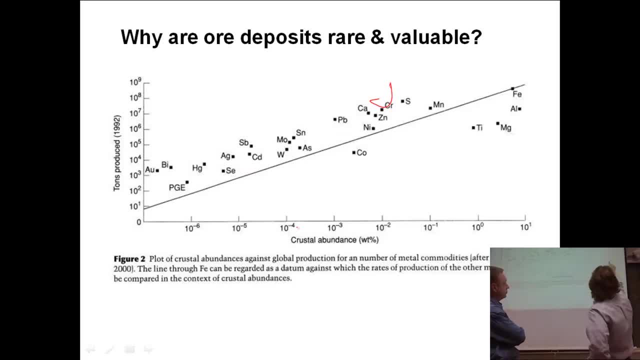 line and we can see that something like iron is really really abundant, like right over there. and then we can look over here and compare it to gold we're just talking about for that TV show, and that's not very abundant at all. it's pretty rare, right, and but we're looking at tons produced in 1992. so you know you. 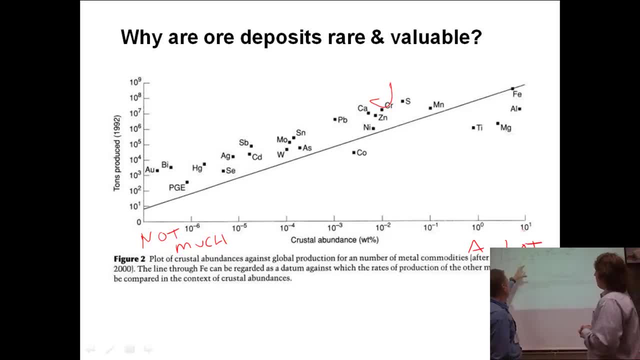 can get an idea of the what we're producing, what's important to us, what's the most valuable resources, those things over the top, those are the things that that's going to give you a more bang for your buck. those, yeah, those are the things that were. these are the resources we're shooting for a lot of the time. 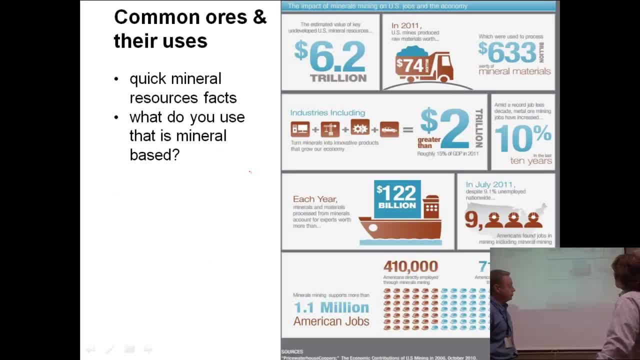 mm-hmm. common ores and their uses. this slide, this would be one that we're probably gonna break out in class and you get a lot more in detail. so you know, at this point, I think, get an overview of what's on there. but you know, it's, this is just filled with. 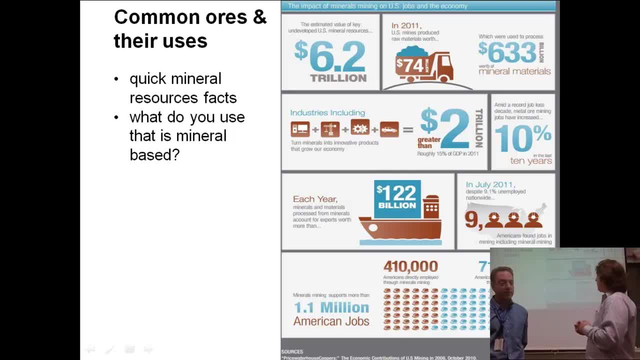 those quick mineral resources and facts. it says: what do you use that is mineral based? so it gets back to our question that we already had is: what are minerals used to make? yeah, and they can click on this from here as well. so you can go ahead and click on this if you want to go ahead and explore now, if you have. 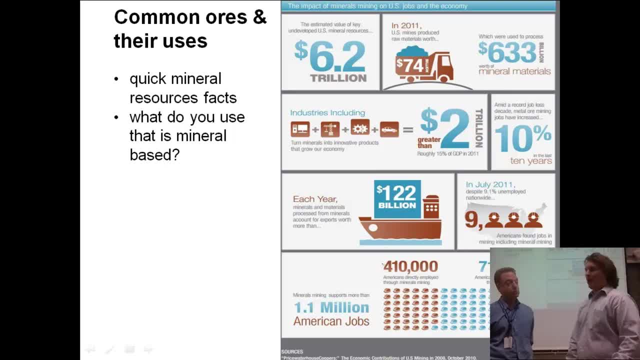 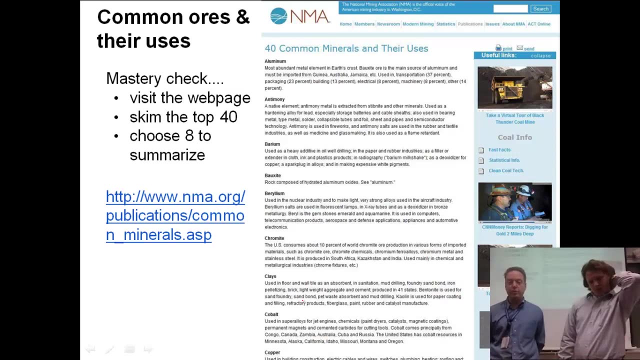 some time, but we are going to be doing it in class and it brings up a lot of different things too about, especially about, about jobs and what that means too. so there's a lot of other impacts that it has on society overall as a whole. definitely so common ores and their uses, so mastery check. so 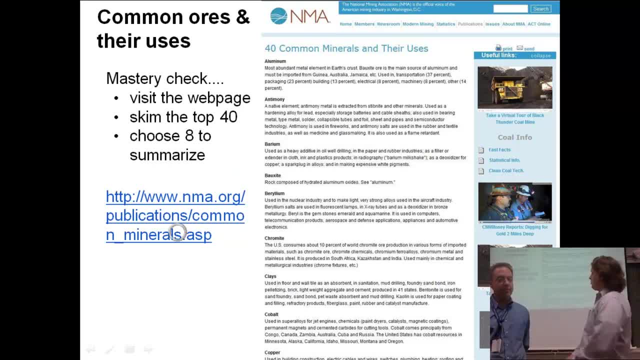 visit the webpage, skim the top 40 and choose 8. to summarize, so they're looking at basically the different ores, sure? so go through the whole list. I wouldn't pick what the first. you know eight or something like that. pick ones that somehow you think are kind of interesting, uh-huh, and choose eight and you're gonna. 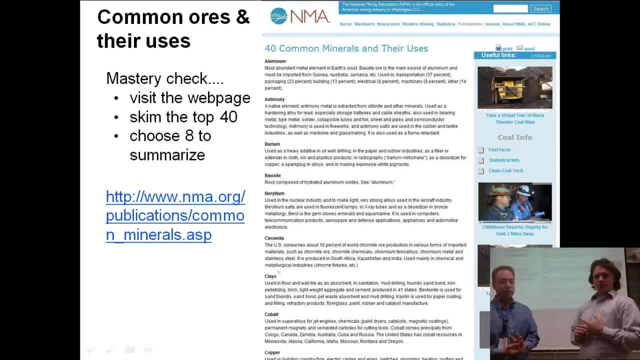 summarize: what did the, what is the common or and what are the uses? how do we use them? information that's important and relevant. yeah, exactly all right, and that is the end of the first segment. excellent, all right. thanks a lot, mr Ben. 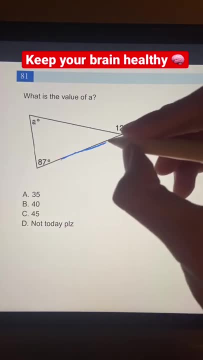 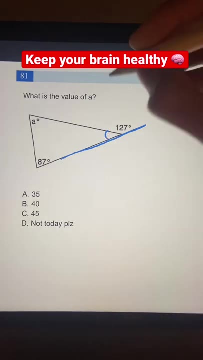 What is the value of A? So the first thing you should do when you see any type of problem like this is locate straight lines, because in any straight line, all of the angles added up has to equal 180 degrees. So to find this angle, all we have to do is take 180 minus 127 and we're going. 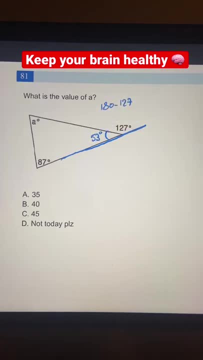 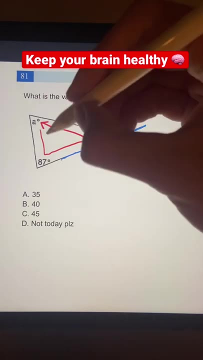 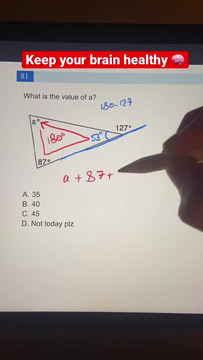 to get an angle of about 53 degrees. Okay, so now we're almost done. Now the next step is to know that in any triangle, all the angles inside the triangle has to add up 280 degrees. So what that means is that A plus 87 plus 53 has to add up to 180 degrees. So 87 plus 53 is going to be 140.